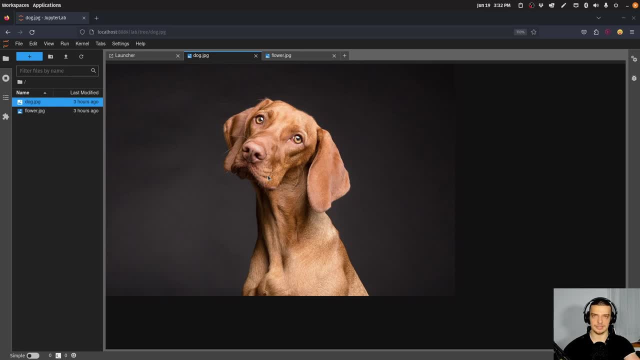 image would be reduced down to the two most important colors of this image. So, for example, in this case, most likely it would be the dark gray background and the gold brown foreground. So we would lose a lot of detail because we would end up with two clusters, meaning two colors in. 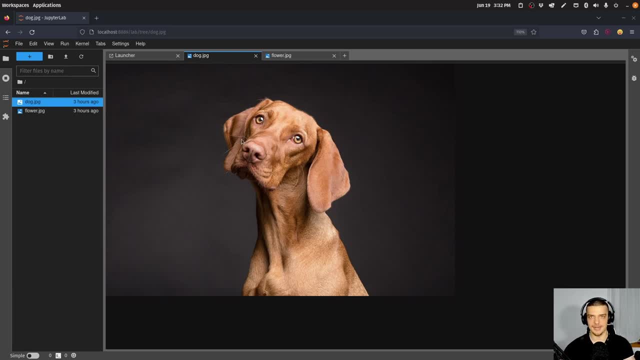 every single pixel In this image will be assigned to either cluster A or cluster B, And of course, I can do the same thing with three clusters, four clusters, five clusters and so on, And the more clusters I have, the more colors I have, and the more colors I have, the more details I have. And you might be. 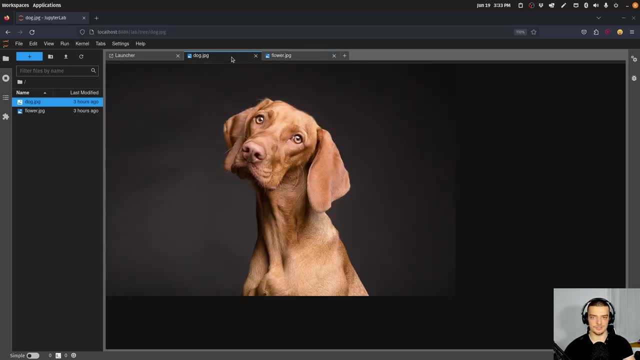 asking: now: okay, why do this in the first place? Why would I want to cluster an image so that I can lose quality? You can have a number of different reasons for which you want to do that. So first of all, you could do this as a pre-processing step for computer vision tasks. 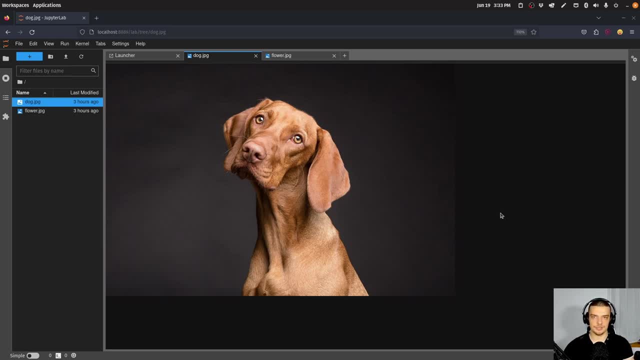 So, for example, you could say I want to perform object detection or any other computer vision task where I need more simplicity, And instead of feeding the detailed pixels into the algorithm, I want to have a very basic version with five colors where I have the most important distinctions. 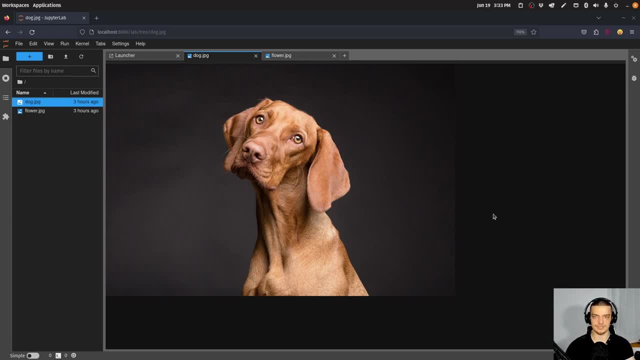 being made. but I don't need all the photorealistic details. I just need the basic outlines and the basic colors. That would be one way or one reason to do this. The other reason would be, for example, to just compress the image. So if you use not five clusters- 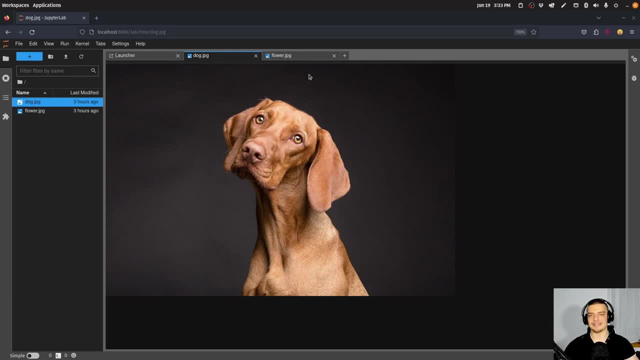 but maybe 50 or 70 clusters, you would get an acceptable level of detail for a couple of images and you would need less megabytes or kilobytes to store the image because you have less detail. But still, sometimes, if you use enough clusters, you won't even notice the difference. So this is 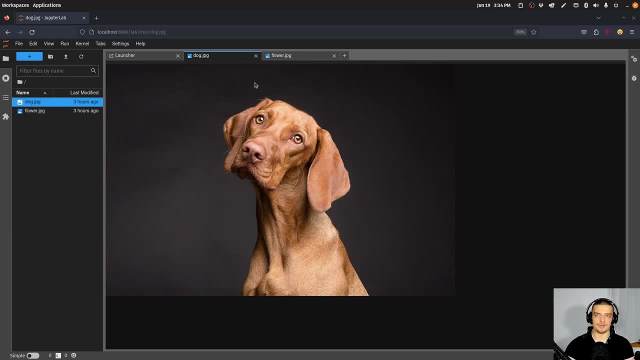 why we do that. Now let's talk just briefly a little bit about how we do that on a theoretical level. I'm not going to go into the details of K-means clustering because I plan to do that in a video: K-means clustering from scratch. in the same way I did it for regression and for. 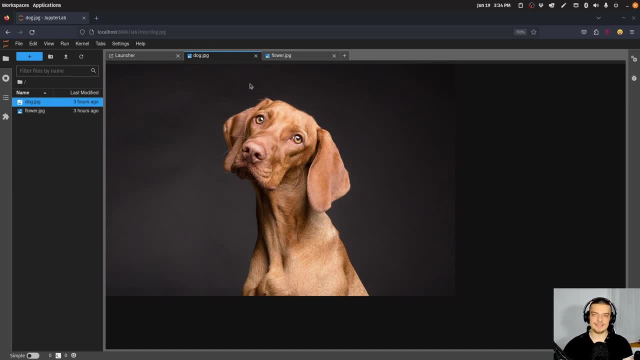 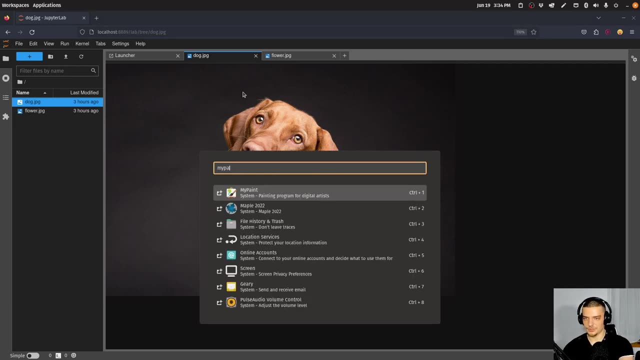 K-neighbors classification. But I want to give you at least a very basic understanding, a theoretical understanding and intuition: what is happening behind the scenes- And for this I'm going to use my paint here And in general, when you use K-means clustering. 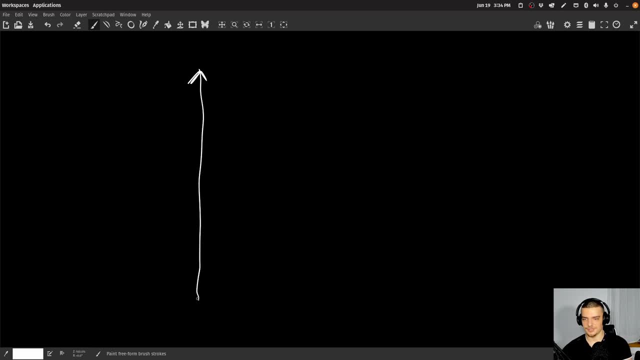 what you have is you have a coordinate system. Now, this is not going to be a beautiful coordinate system. In this case, let's say, we have two-dimensional data, So every data point is x and y, an xy tuple. So a point in 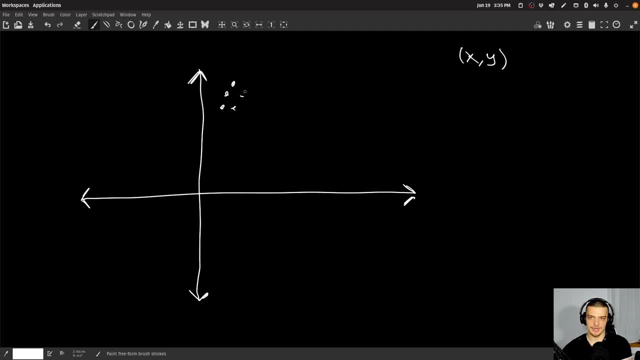 a coordinate system. And now let's say, I have a bunch of data points here and a bunch of data points here and a bunch of data points here, And then what I want to do is I want to say, okay, I don't have any labels for those, So this is not a classification task. I don't know that this is. 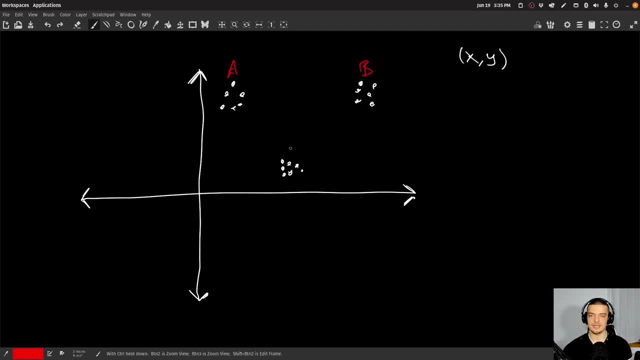 class A and this is class B and this is class C or anything. Those are just raw, unlabeled data points And what I can do now with K-means clustering- and I'm not going to go into the details of how this works, especially also because I have a video actually on K-means clustering and what it does- 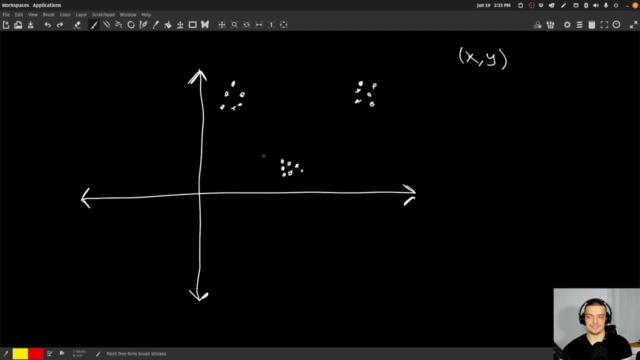 and how to use it in Python. Essentially, you can think about this as finding the centers of gravity here. So you have, let's say we want to say n clusters. in this case is three, So we want to have three clusters. Go ahead and find the best three clusters And then we would just initialize. 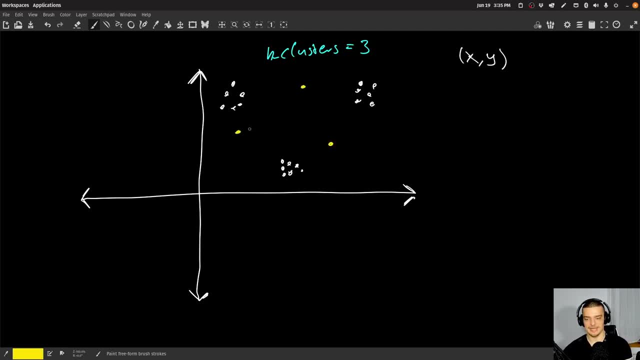 some random Points here, being the centroids for the clusters, And then, through a couple of iterations, through the K-means algorithm, we would end up somewhere here in the cluster middles with those centroids and it would find these clusters. Now, when you run it again, you might end up with different. 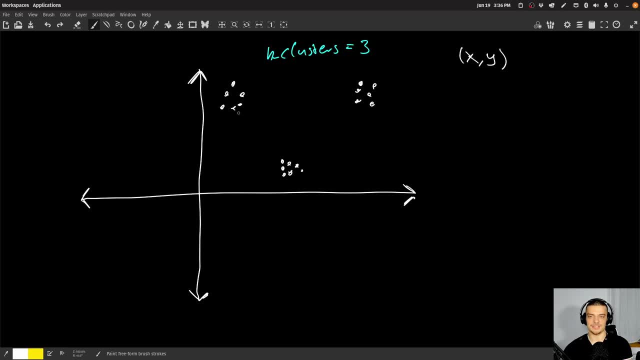 clusters, especially because real data doesn't look like this, but it's oftentimes very unclear. So in this case, it's very easy to spot the three clusters. We have this one, we have this one, we have this one, And it's very, very easy to say that there are. 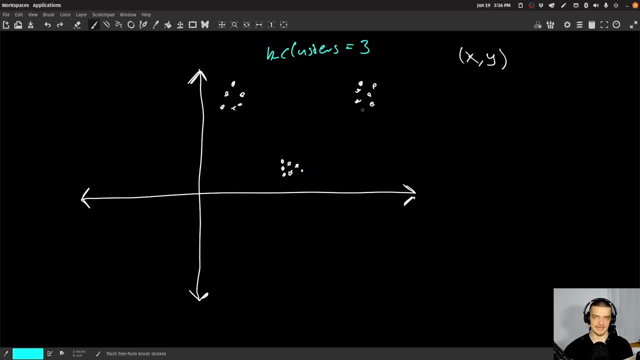 quite distinct. Now, this is the basic idea of clustering, finding groups that belong together. Now, how is this relevant for image segmentation? Very simple, Let's say we have now an image of I don't know some person here, And of course we would have. I didn't want to start down, let me 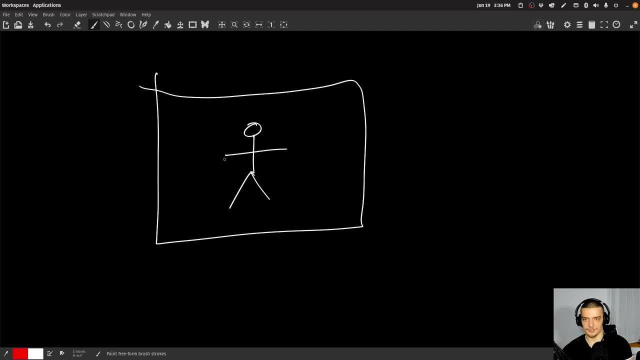 just go back. Let's have different colors here. So maybe I have a red sword and maybe I have a banana in this hand. I don't know. maybe I have a blue hat or something. This image would contain pixels, So it would be. 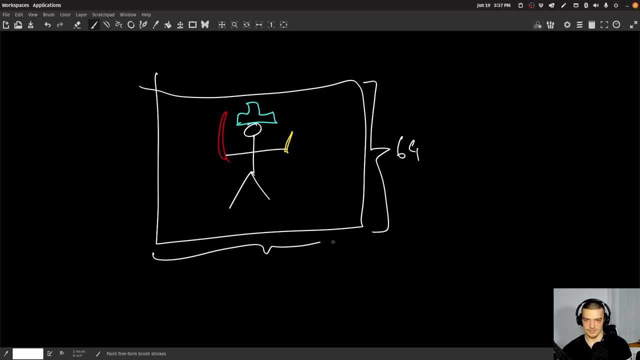 for example, let's say 64 times 64 pixels, And these pixels have three values. So we would have RGB, for example, red green blue. every single pixel has red green blue. So you could also say: 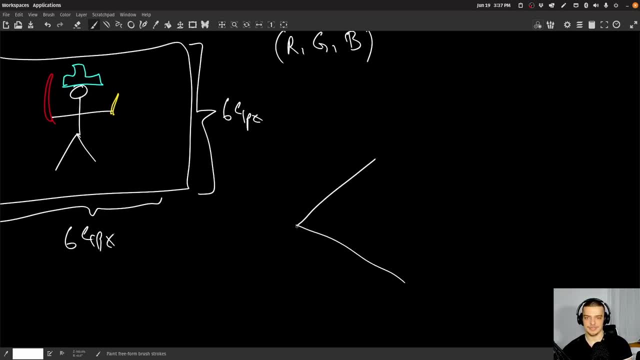 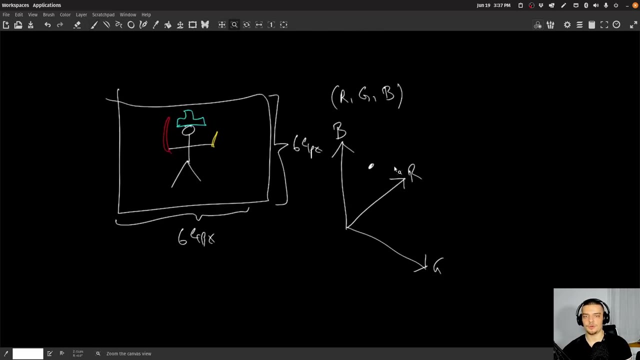 using different language at every pixel is, in a sense, a point in three dimensional space. So you would have R, G, B, and every pixel is some point in space. Now, what we want to do now is we want to take all the pixels and we want to cluster them. 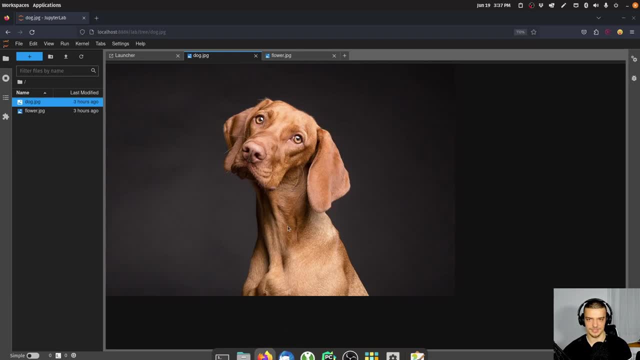 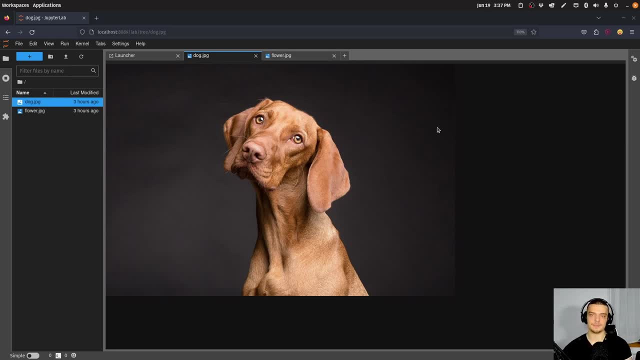 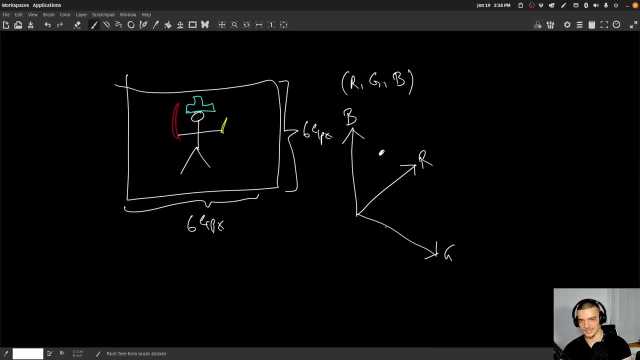 light gray and dark gray and black pixels would probably be quite similar, would be quite close together mathematically. Speaking of the Euclidean distance, this is what we use in K-means, clustering, basically just the Pythagorean theorem. distance is what I sometimes like to call it. So basically, 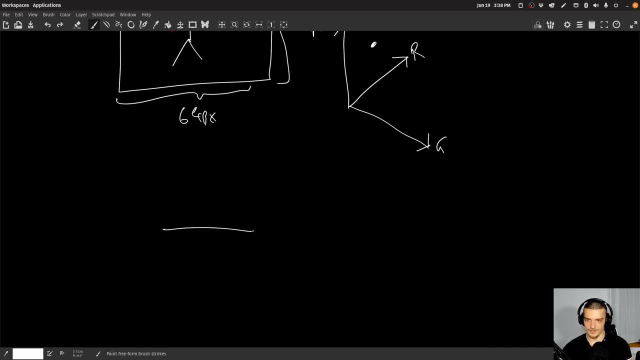 you just say, if I have, if I move into the X direction a certain number, if I move into the Y direction a certain number, this here would be the Euclidean distance. So the square root of X squared plus Y squared. But I said I don't want to go too much into the mathematics. 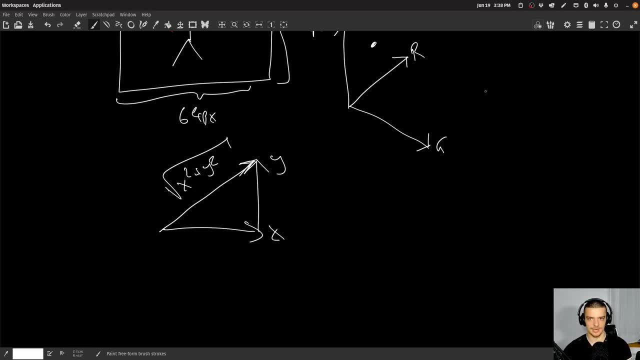 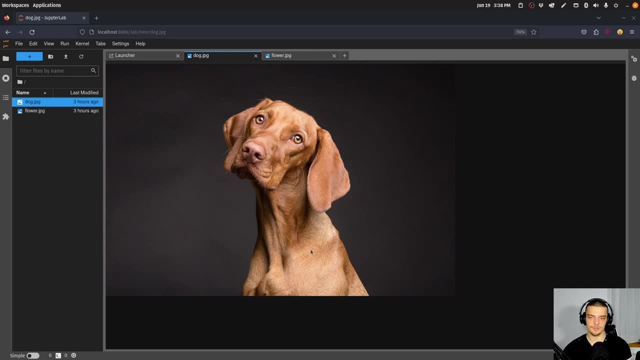 This works also for N dimension, doesn't work only for X and Y. it works for X, Y, Z and for 50 dimensions as well. But in this case what we would do is we would take every pixel and we would compare the pixels And we would say: okay, those are quite similar And those are quite similar. So 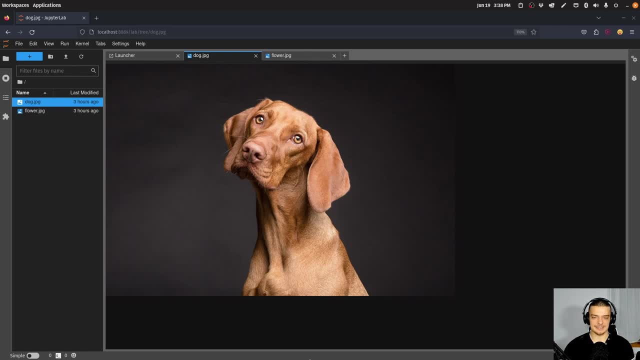 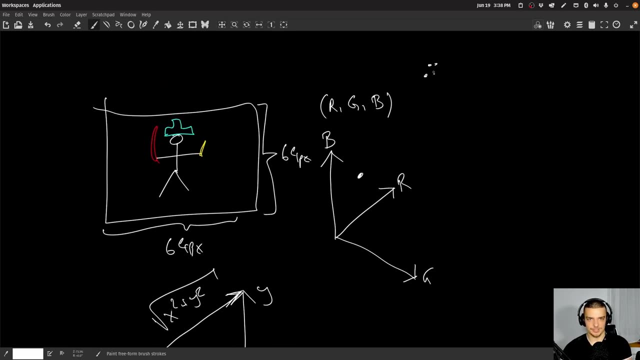 we have the two classes, And these two classes have a centroid, the center of gravity that we talked about previously. So if I have a bunch of pixels here and a bunch of pixels here, what I'm going to do is I'm going to 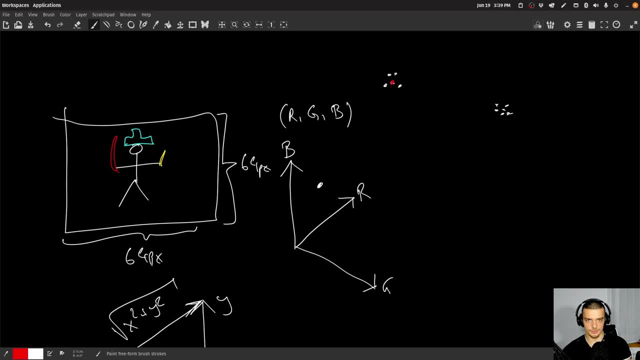 reduce all of them to the same color. So all of those are going to be this And all of those are going to be this. Now, this is not red and yellow. this is the center of gravity of this class cluster, And this is the center of gravity of this cluster. So maybe you have here some gold. 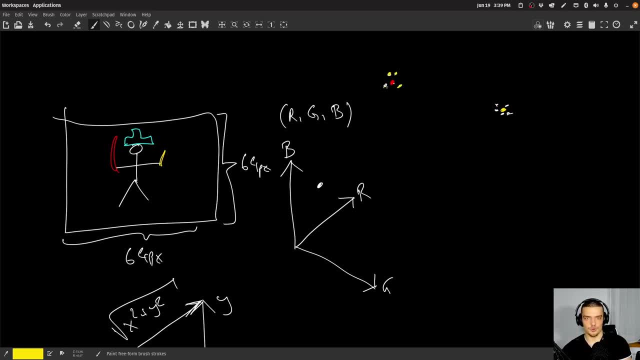 brown, some brown, some gold, some orange or something. all of this will be reduced to this one color here, And of course, the more clusters we have, the more different colors we have, the more different centroids we have. That's the theory. 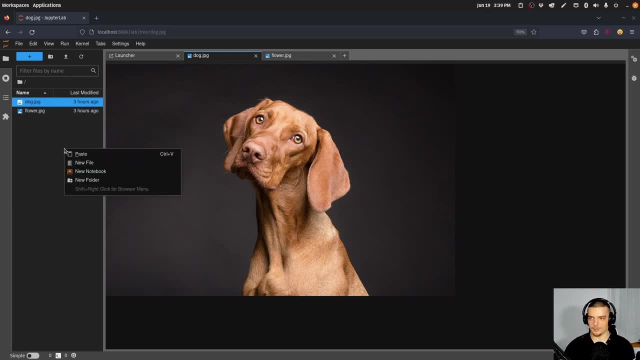 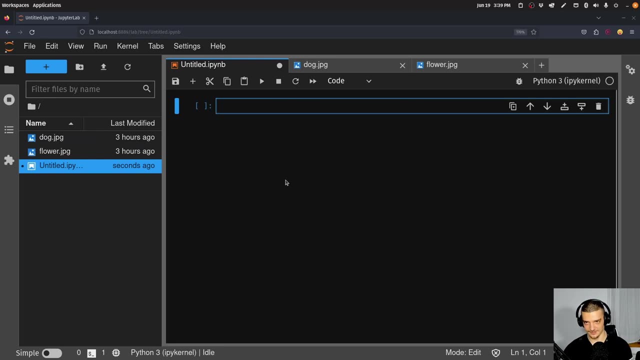 Now I hope this was not too boring or complicated for some of you. So let us get now into the code where things are going to be easier, because we don't really have to do any of that stuff manually. we can just call the k-means clustering. It's not a classifier, So the k-means algorithm we can. 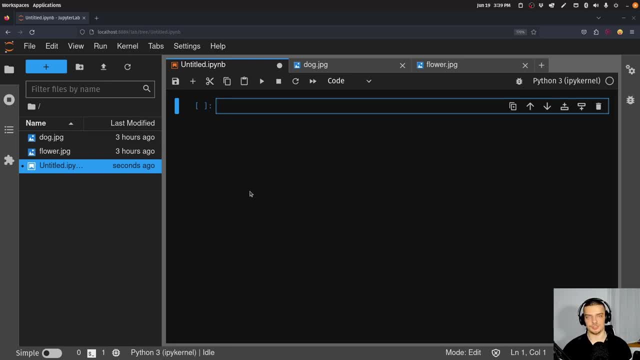 create an instance and we can do the clustering on the data, which is the image, and then we can see what the segmented image looks like. So we're going to start by saying: import matplot lip as MPL And import matplot lip dot piplot SPLT. 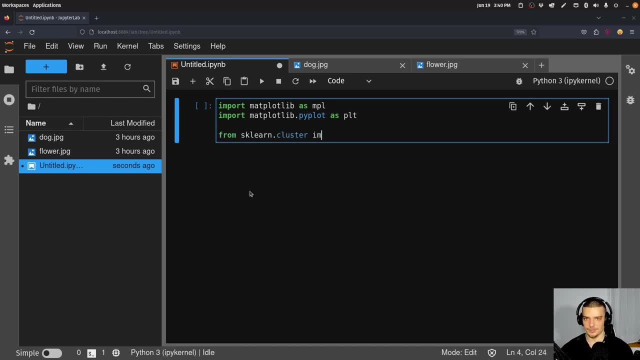 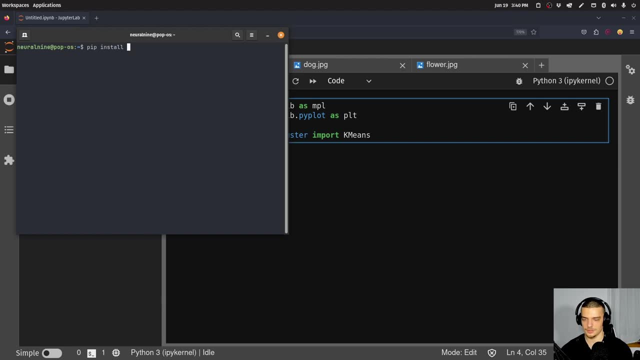 And then from sklearn dot cluster we want to import k-means And, of course, if you don't have these installed, pip or pip three install scikit, dash learn and matplot lip. Those are the two packages that you need And later on, for the outputting of the compressed images, we're going. 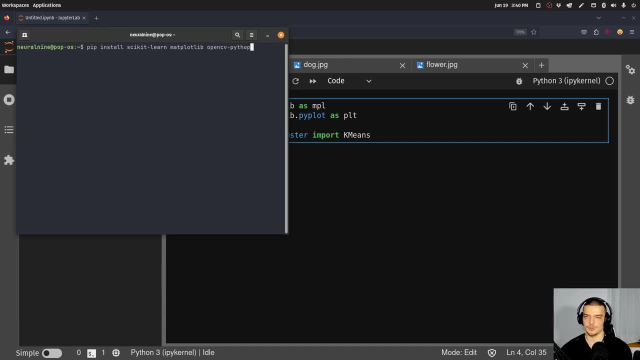 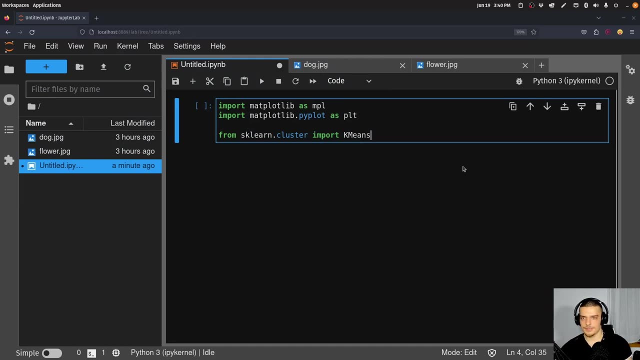 to also use OpenCV, dash Python. So install these three packages for the video today. Those are the installs, So those are the imports, And now what we're going to do is we're just going to load our image, for example, the doctor JPEG, by saying: image equals MPL dot. image dot em read. 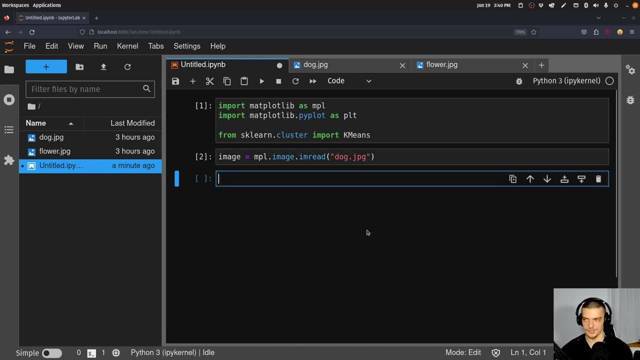 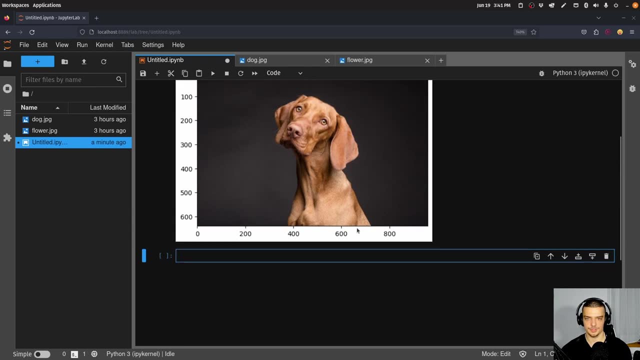 Doc, dot jpg. And then we can just say PLT, dot M, show image to display the image in this Jupyter notebook. here you can see this is the doc And we can also look at the shape. So if we say image, dot, shape, 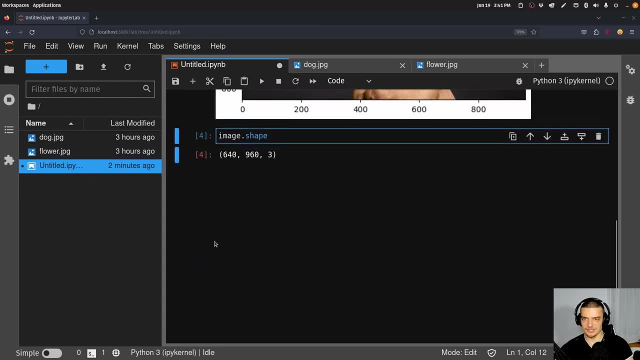 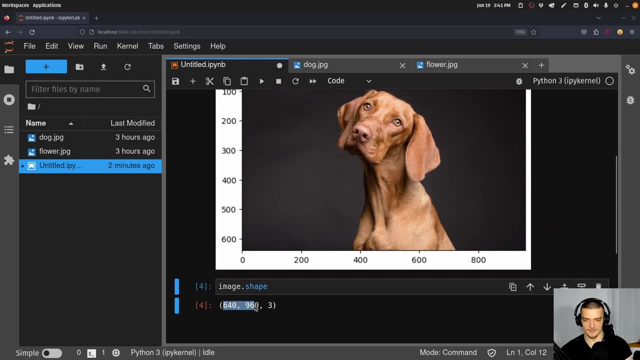 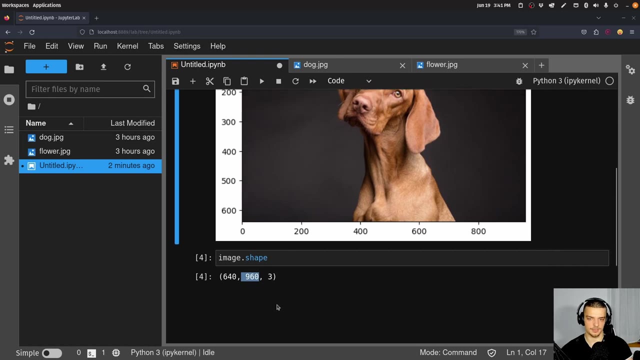 and we run this, you can see that it is 640 times 960, with three dimensions being RGB, the three colors. So we have this many pixels here, So we can see that it is 640 times 960.. All of these pixels are three dimensional data points. as we 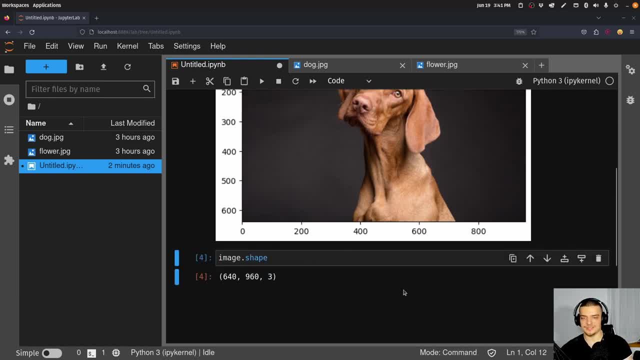 can see here. And what we want to do now is want to take that data, we want to flatten it, at least these two dimensions. you want to make them into just a bunch of different pixels with three different coordinates. And then we want to use k means clustering- to cluster the individual pixels. 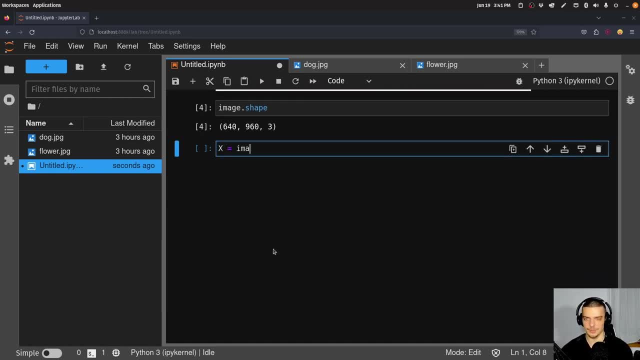 So what we're going to do is we're going to say x is going to be equal to image dot reshape, And now we're going to use negative one to basically combine these two into into one dimension, into one axis, And then we're going to keep three. So now, if I say x, dot shape, 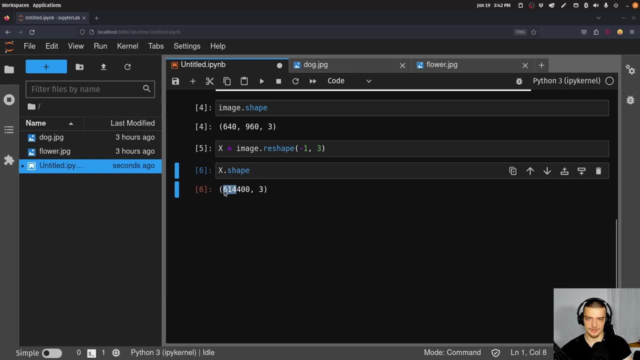 we can see it's 614,400 pixels, with three coordinates, with three values, RGB, And what we want to do now is we want to just use k means. so we're going to say k means equals, k means n clusters. We're going to start with two so that you can see what we were talking. 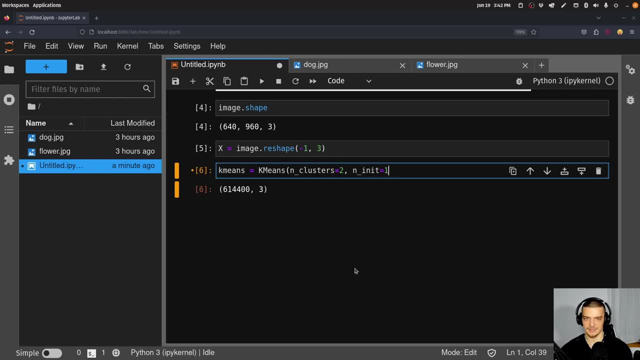 about all the time, And then we're going to also say n in it being equal to 10.. The only reason I said this manually is because if I don't do this, I'm going to get a warning message that I'm not setting the default parameter, or actually I'm not getting the warning message. Okay, so let's just. 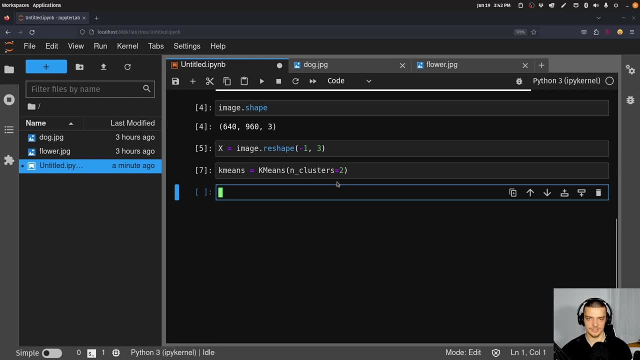 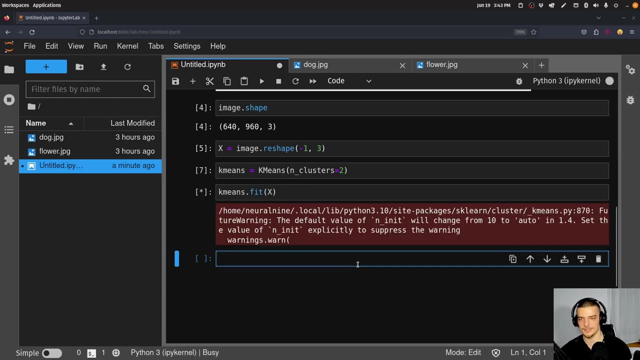 not set. it basically just tells us how many times we're going, how many times we're going to initialize the centroids randomly. We actually get get an actual clustering result. And now we're going to say k means dot, fit, x. Oh, here I get it. Okay, so let's just use it and in it 10, because in future versions it's going to be. 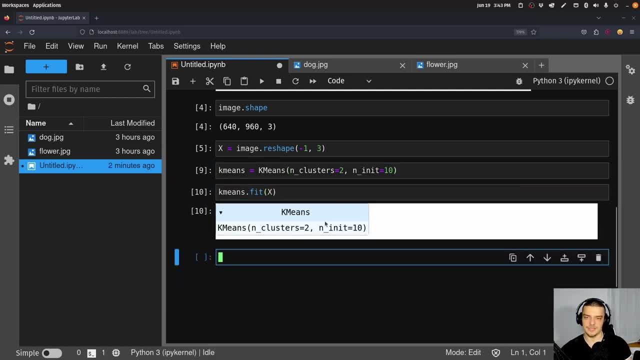 set to auto. But let's just go ahead. k means dot fit x. And then what we're going to do now to actually get the segmented image is we're going to say segmented image is equal to. k means dot cluster centers, underscore, k means dot labels, I think, underscore and then segmented. 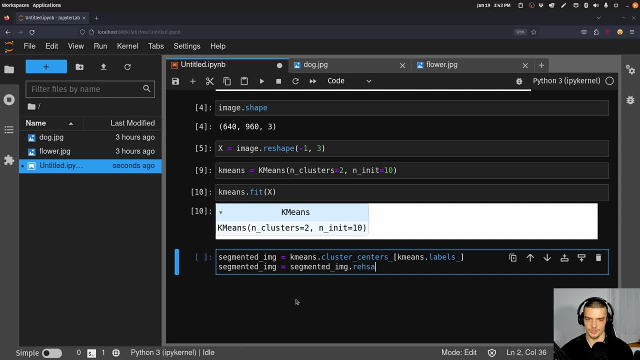 image equals segmented image, dot reshape, And we're going to shape it back into this shape of the image that it had in the first place. And now all we have to do is we need to say PLT in show segmented image and we need to divide by 255. 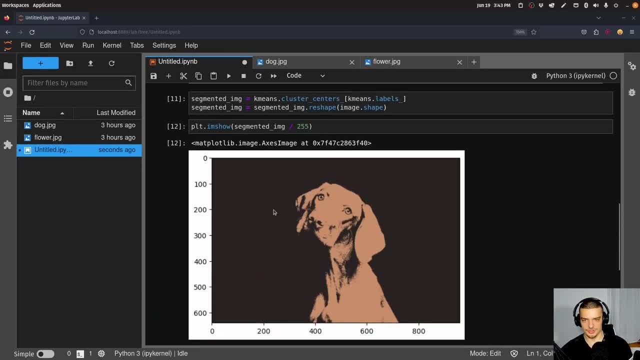 To get values between zero and one. And here you can see what the result of this looks like: exactly what we said. we have two different colors. we have the background, which is kind of dark, gray, almost black, and then we have this gold, brown type of color for the dog itself. So you can see. 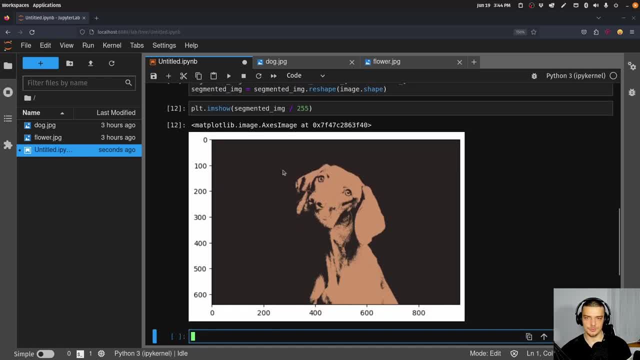 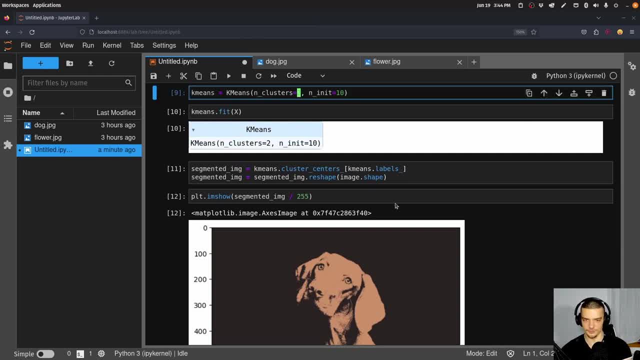 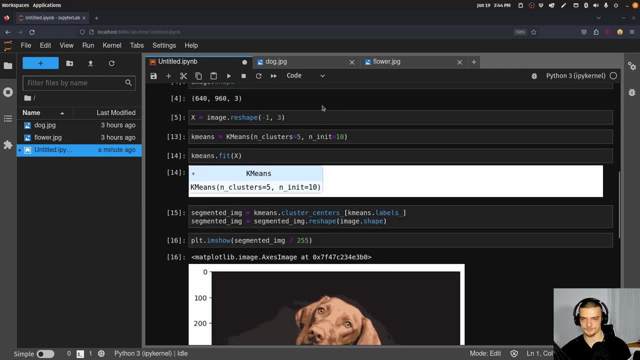 I add here, the more detail I'm going to get in the image. So if I say, for example, give me five clusters, I'm going to get five different colors, meaning more detail, as you can see here, And I can also do this with 50.. I think it's going to take longer, But I can do this with 50 as well. 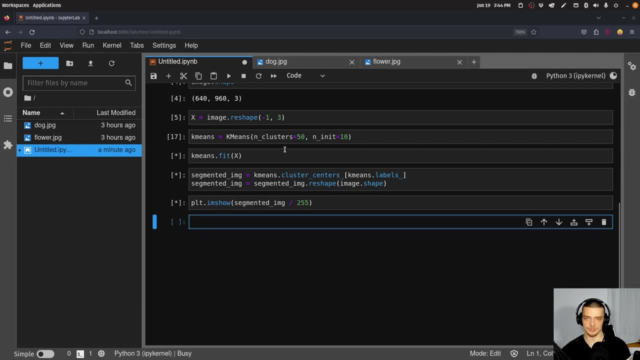 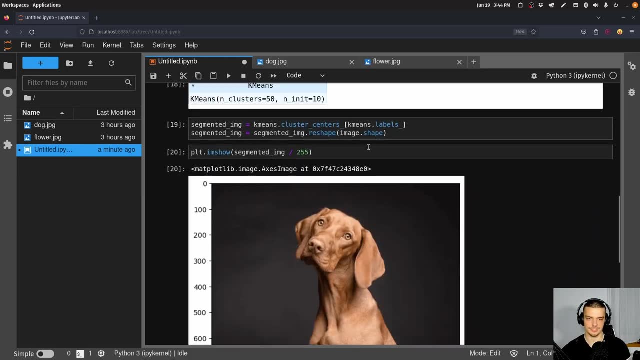 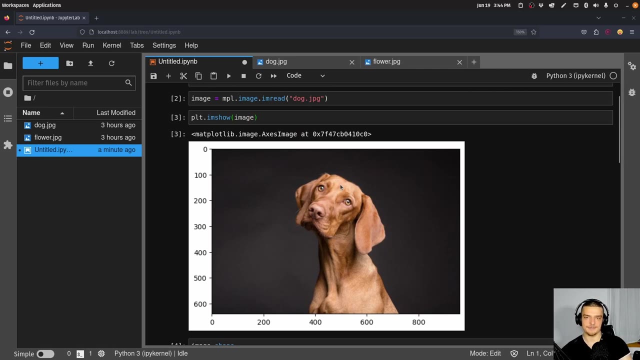 And after some time I'm going to get the image. The more clusters you have, the more time you you will need to run this, the longer you will need to run this, And here you can see that it looks like nothing changed, And I'm not sure if we're going to get a significant compression here. 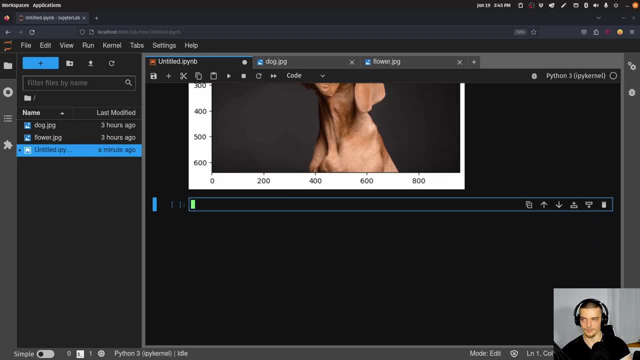 if we write this to an image. So let's just go ahead and try to see what happens. We can basically just say import CV two And we can say CV two in right now. first of all, we need to get the image. 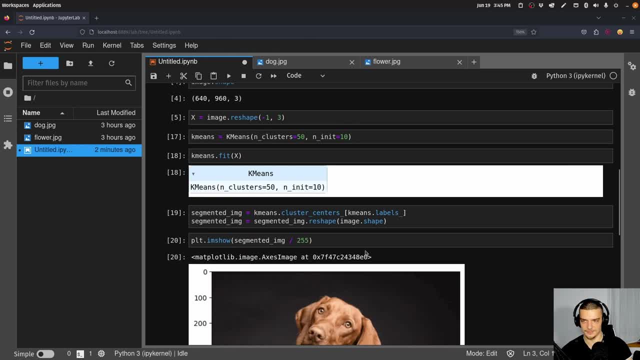 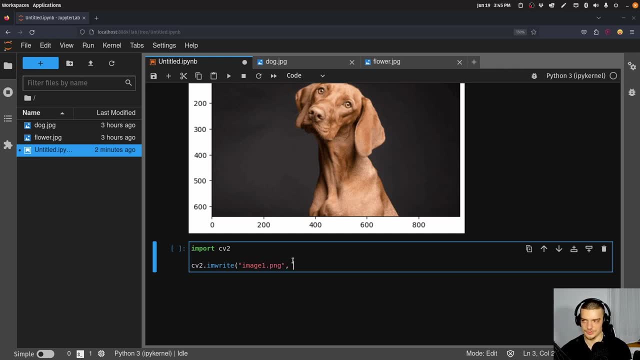 Or actually we we have the image already. So we have image and we have segmented image. So we're going to say image right, Image one dot png, And we're going to use CV two dot convert color Because OpenCV uses the BGR. 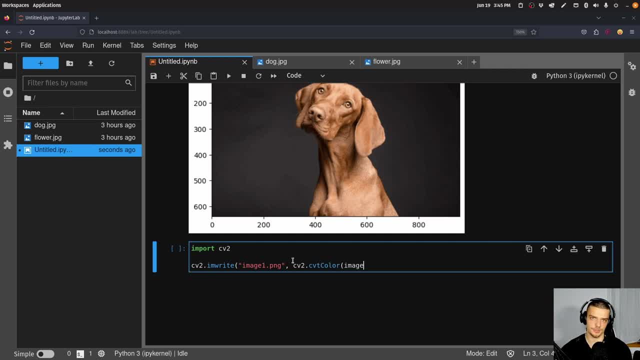 color scheme, So blue, green, red, and we're using RGB which is red, green, blue. So this is just going to be swapped And we're going to have different colors. So we're going to just convert the image to CV, to color underscore, BGR to RGB, And we're going to copy that and we're. 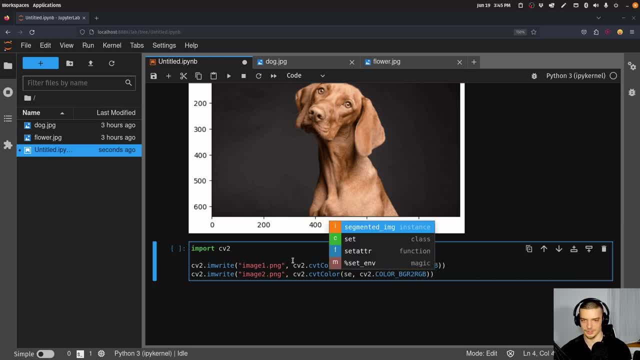 going to sell it in what we call a Direct toバessed borderut, which has the one color number and let's say it is a color, And we're going to go back in here and張We're going to say: let's see what we are going to do. 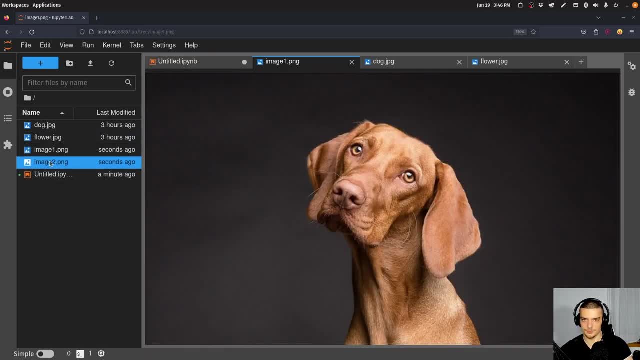 next And we're going to exit the app legal And we're going to� do the same thing for image two and for the segmented image. Now, for the segmented image, we need to say ts type And I think let me just So, we have image one and we have image two And you can see that there is some difference here in. 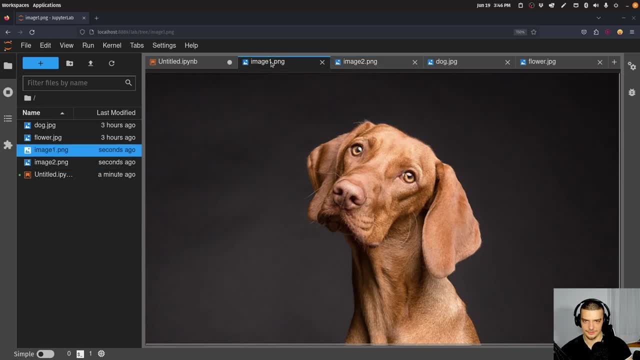 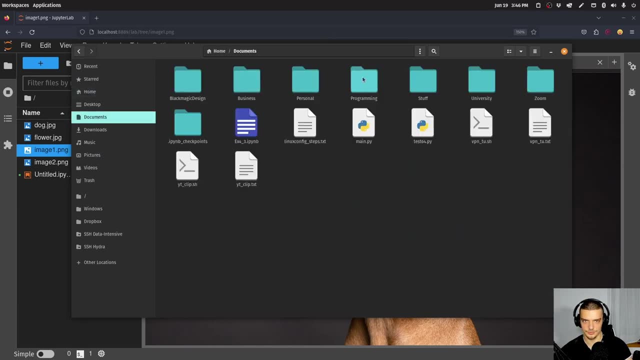 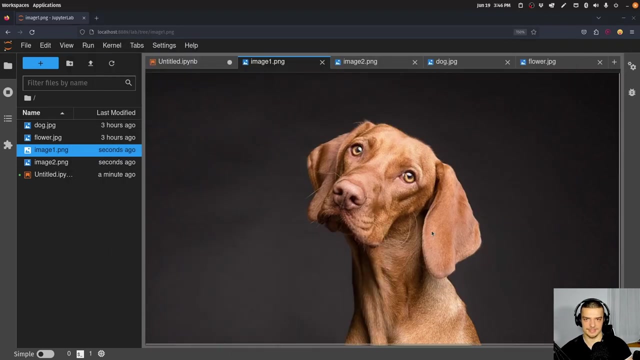 the detail level, but it's not too big. Now let's just see how how much difference in size we have here. So if I go to programming Python current, then we have image one being 622 kilobytes and this one being 417 kilobytes. So a little bit of compression is happening here, And if I 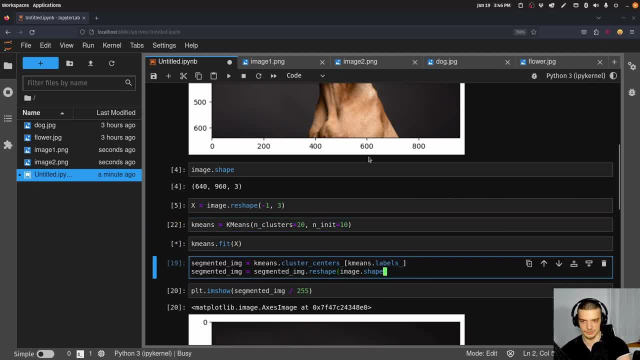 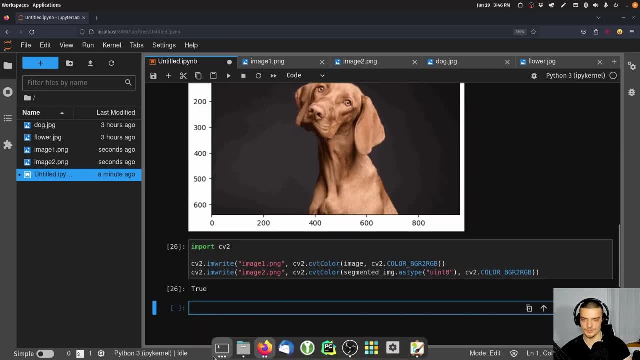 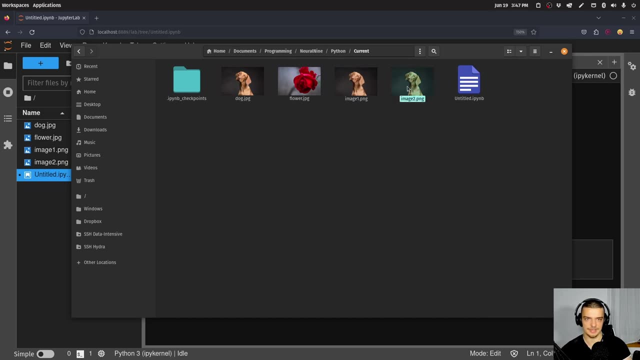 reduce this number here to 20,, for example, then of course we would lose a lot of detail, But you will probably see a larger compression. So we have now 622 and 309.. So less than half of the size. And if we compare, 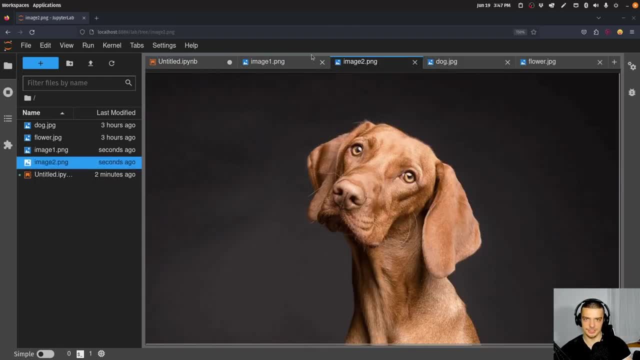 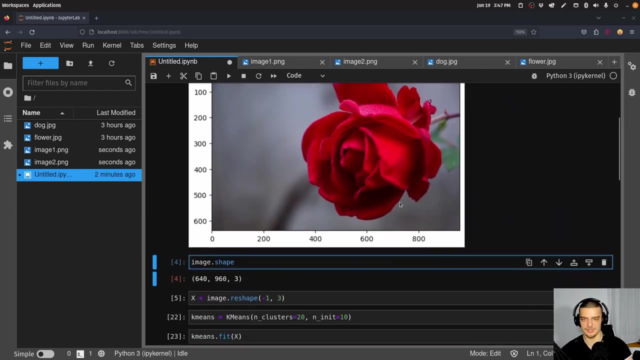 the quality. yeah, you can see that it actually doesn't look too much worse than the previous one. So 20 or 50 doesn't make that much of a difference. However, I think for the flower it's a little bit more clear. So if I go and do the same thing for flower JPEG, then this is the image, And if I 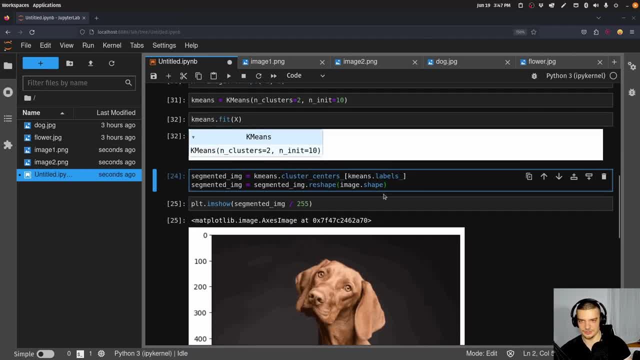 run this now with two. first of all, you're going to see that this doesn't look good at all as far as I remember. There you go, So you don't really see what's happening in the image. Now I think. 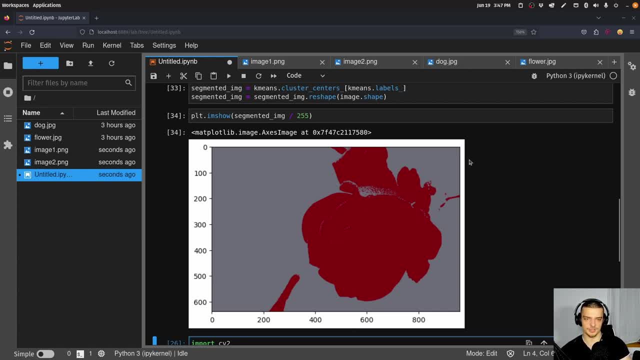 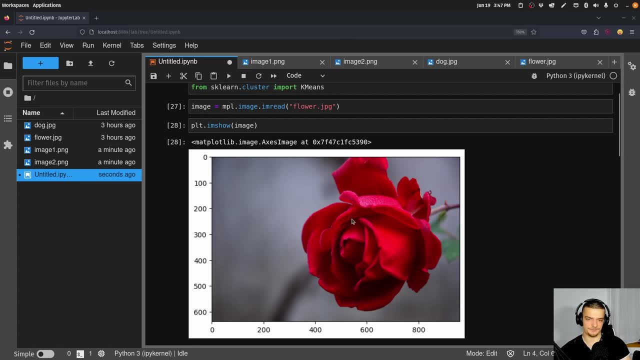 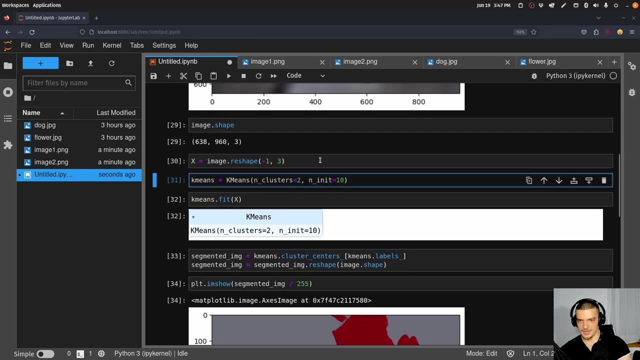 I think that this is even too little for in for for an object detection, because the thing about the rose is it's not enough to just get the shape, you need to get a different, different types of red, because otherwise you don't see the structure here. But if I change this maybe to 10, we should 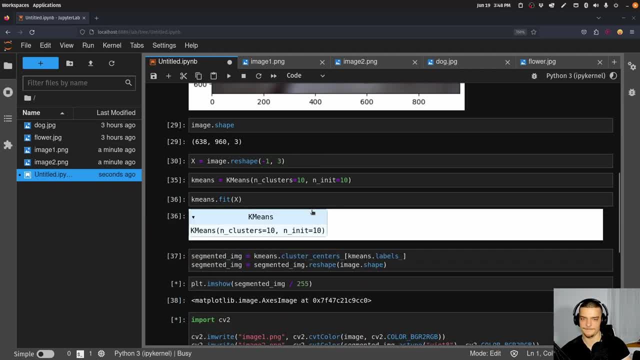 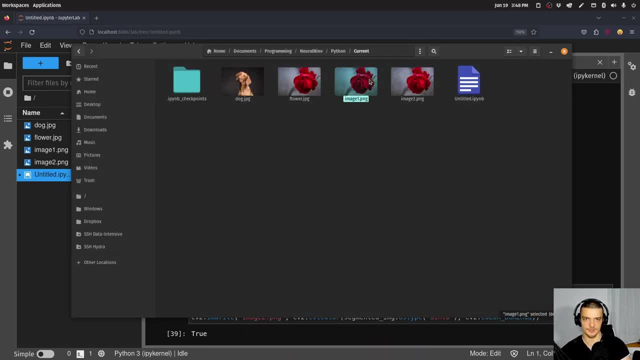 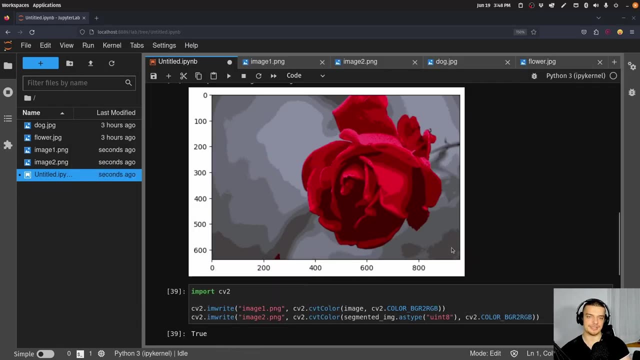 get something that looks a little bit better. Yeah, I mean, you can at least see it's a rose now, And maybe an object detection algorithm will be satisfied with that. But here you can see 600. And here you can see 97. So this is much smaller, But usually this is not.